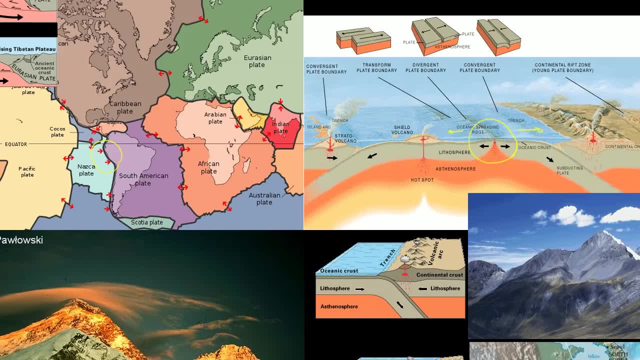 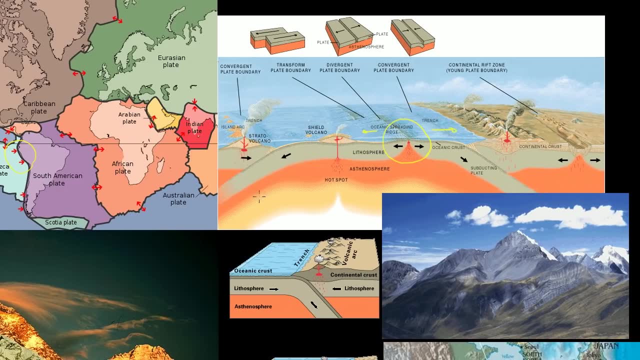 They're running into each other. So what happens over there? So what we're going to do is just go through the different scenarios. The general idea is that one plate is going to get subducted under another. They're ramming into each other. One is going to get essentially pushed under the 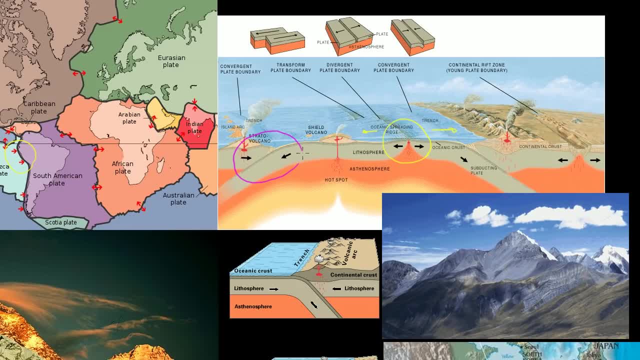 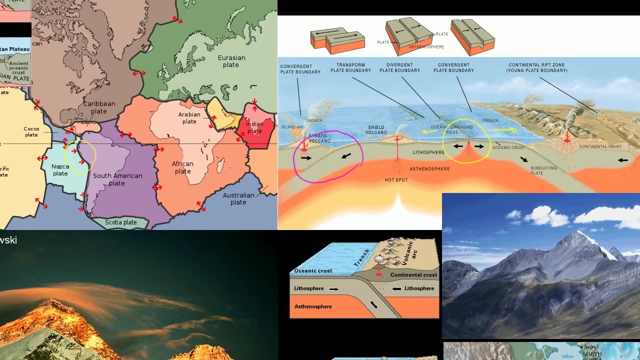 other one. This diagram shows some subduction over here. This is a essentially oceanic plate being subducted under another oceanic plate, So not too different than what might happen where the Pacific plate runs into the Filipino plate right over here, And then on this side of the diagram we see an oceanic plate and the 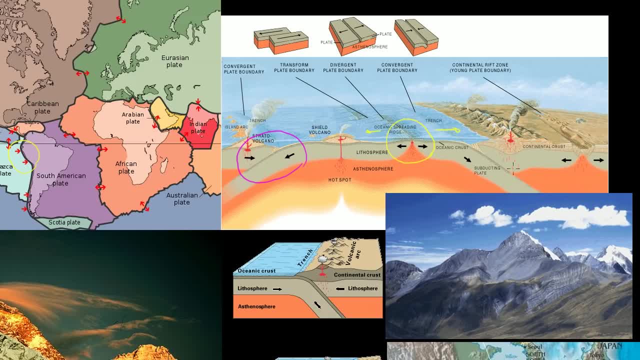 oceanic crust getting subducted under a continental plate right over here. And this is what's happening when the Nazca plate is getting subducted under the South American plate And when that happens, a couple of things, So you have the oceanic plate being pushed under. 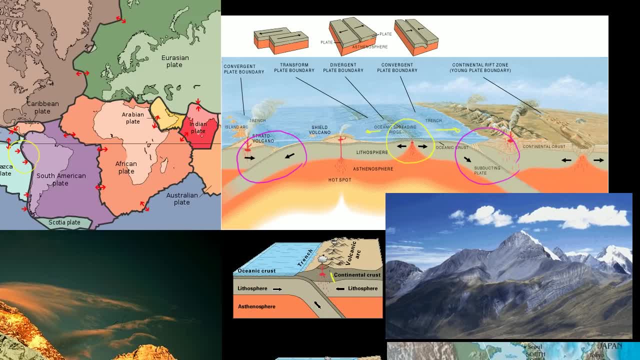 and what happens at the same time, the continental plate gets pushed upwards, causing mountain ranges like the Andes. and that's exactly what causes what has created the Andes is that upward force from the Nazca plate being pushed under the South American plate at that coastline. 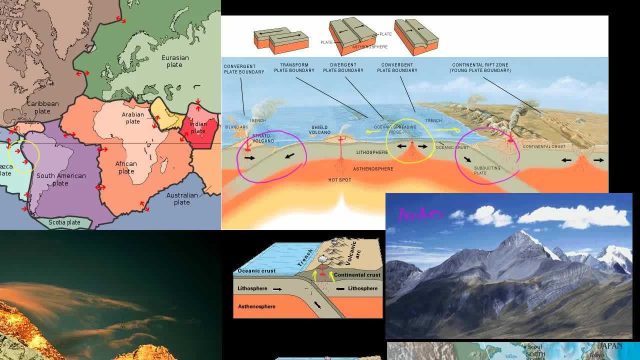 What you're also going to see is- and you can imagine, you have these huge plates grinding past each other and it's not a very smooth process. Every now and then, you kind of reach a breaking point, Huge amounts of energy and huge amounts of energy get released. So you're also going to see a lot of 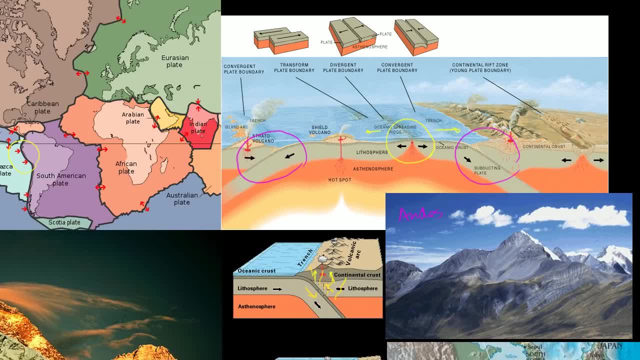 earthquakes in those areas- and you can, and we know that Chile has a lot of earthquakes- And then, on top of that, this is going to result in a lot of heat and a lot of the friction of the plates grinding past each other, essentially allowing magma to form at that part of the rock, because 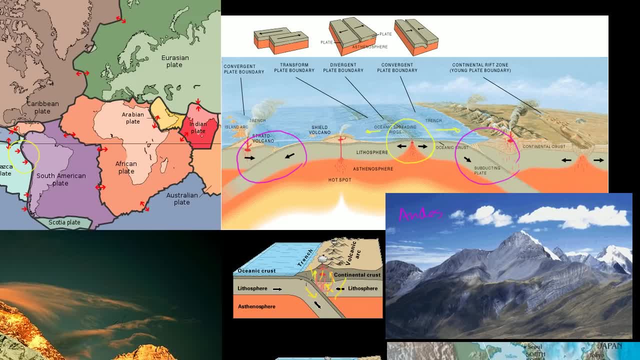 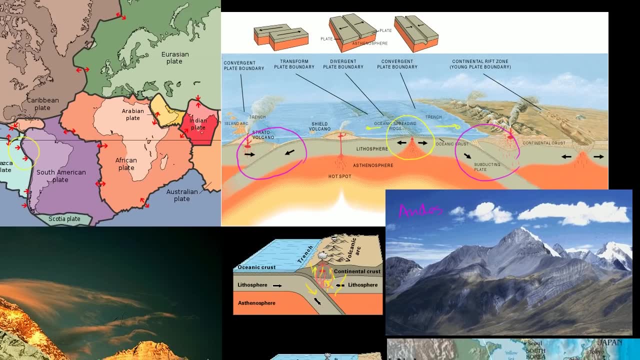 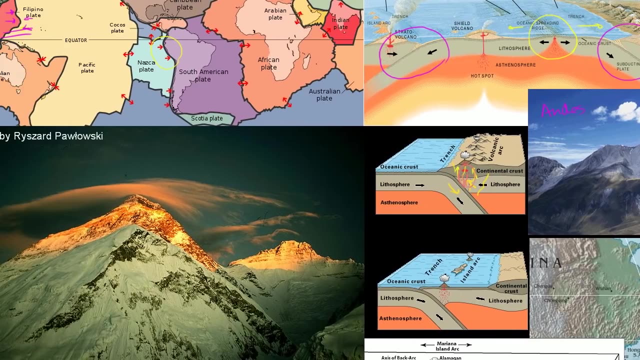 it's getting so heated And so you'll also have volcanoes in these areas where, essentially, something is being subducted Underneath a continental plate. Now we also talked about what's happening in the Pacific, where we have the Pacific plate being subducted under the Filipino plate. That's what we kept keep referring. 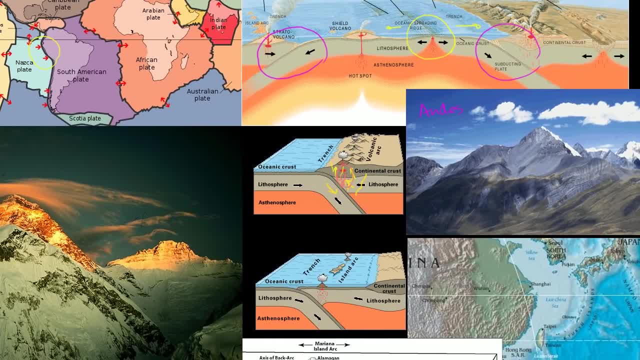 to over here And that's doing a couple of interesting things. Whenever you have subduction, you have trenches. but it's most interesting- or at least in my mind- the deepest trenches have been created where you have an oceanic plate being subducted under another oceanic plate. 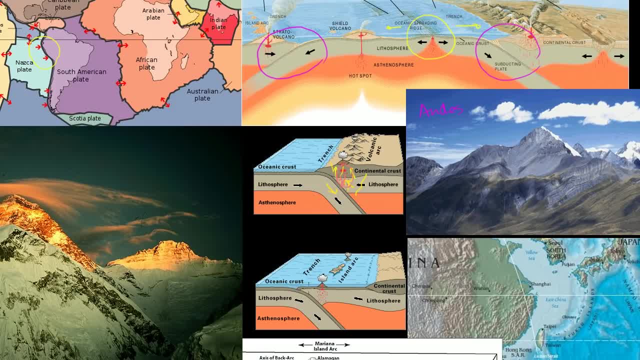 So a couple of things are going to happen. You're going to have a very deep. you're going to have trenches form. You're going to have a trench form over here. we see in this diagram, we also have a trench in the first example, but you have trenches form where the 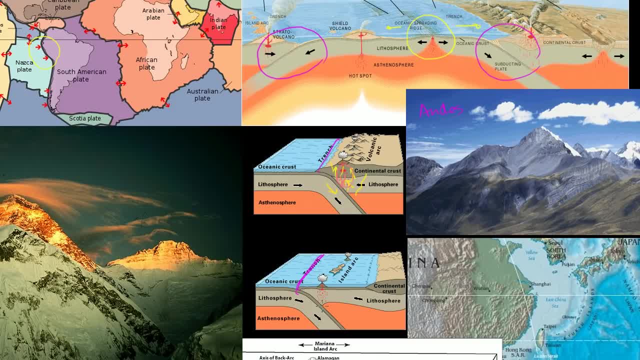 oceanic, where one oceanic plate is being subducted under another and then you have that same type of friction that you saw over here, create volcanoes, and those volcanoes will initially be underwater volcanoes, since these are both oceanic plates, or they were kind of. we're dealing with oceanic crust. 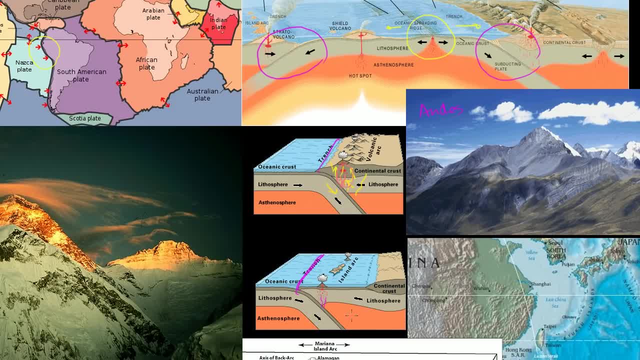 at that point of the plate- it doesn't have to be entirely an oceanic plate- and they'll first be subducted under another and then they'll eventually turn into a group of islands. but as the lava piles up and hardens, it'll eventually turn into a group of islands, and we have that happening where the 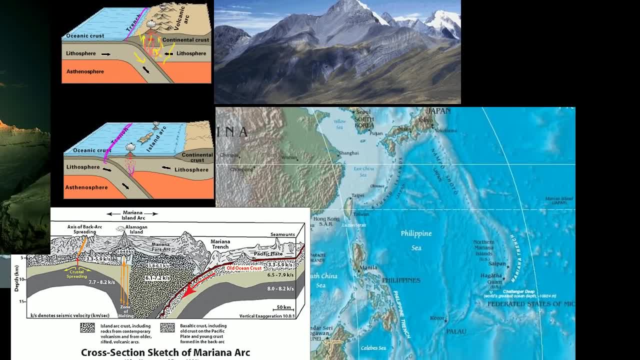 pacific plate runs into the filipino plate, and first we have the trench, so let me just draw everything right here. so this is the boundary, roughly, roughly speaking. this is the boundary between the two plates. this is the pacific plate and this is the filipino plate, right over here and 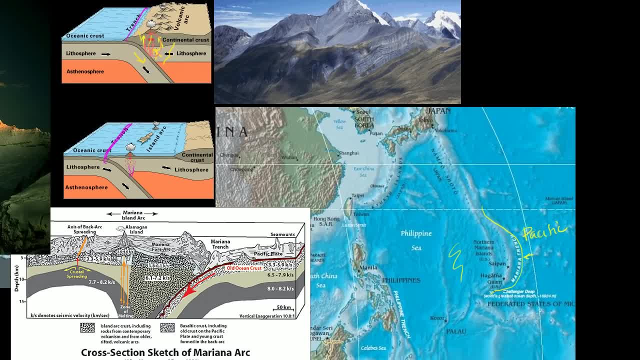 so where it's being subducted, you have the mariana trench, which is the deepest trench in the world. it goes down 11. it goes down 11 kilometers, 11 000 meters. that's deeper than mount everest is high. mount everest is about 9 000 meters high and we'll see that's also due to another convergent plate. 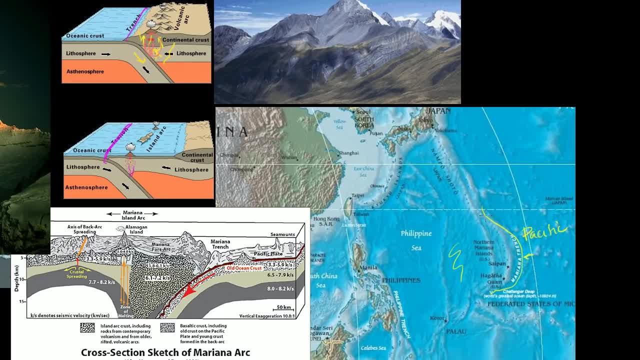 boundary, another place where plates are running into each other. so not only do you see the mariana trench here, because one plate is being subducted under the other, you see the formation of the mariana islands, which are essentially created from underwater volcanoes. because of all of the 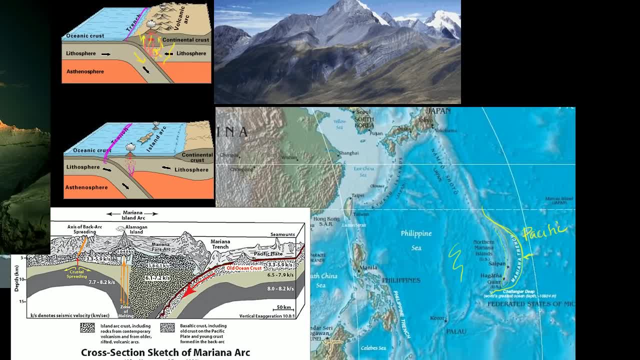 energy being released, and this is actually a depiction of what's the subduction that's happening at the mariana trench. you have this subduction over here and then you have the mariana islands being created by, essentially, the energy causing a magma and lava. uh, essentially. 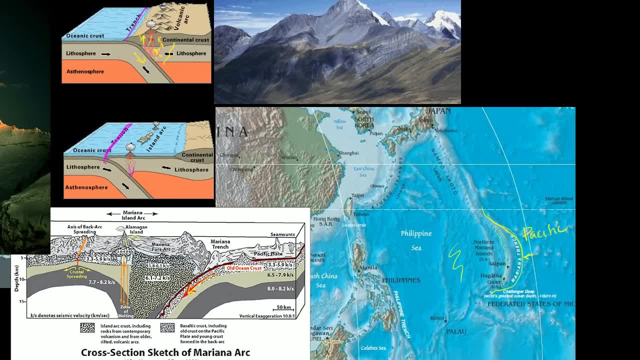 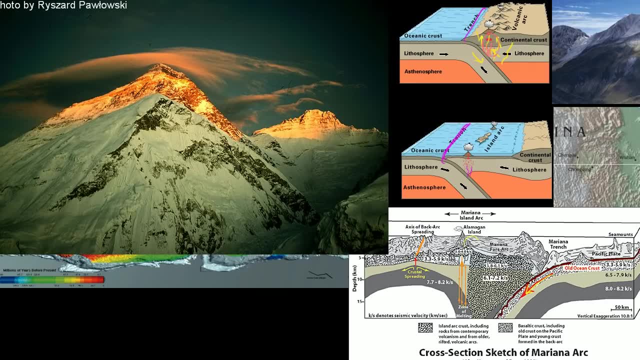 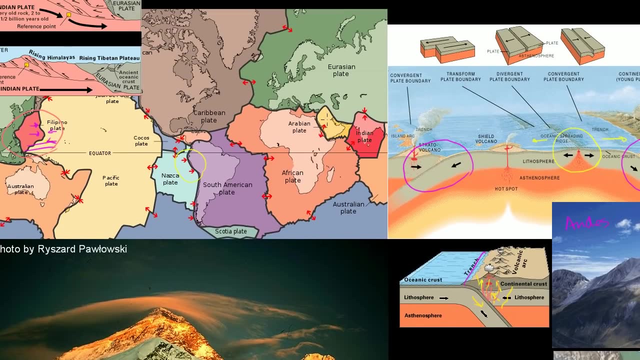 magma before it surfaces, to flow to the top and as lava just goes and starts building these islands. now the last type of convergent boundary is when you have two, two parts of continental crust running. so that's the situation that we have in, where the indian plate is running into the eurasian plate and 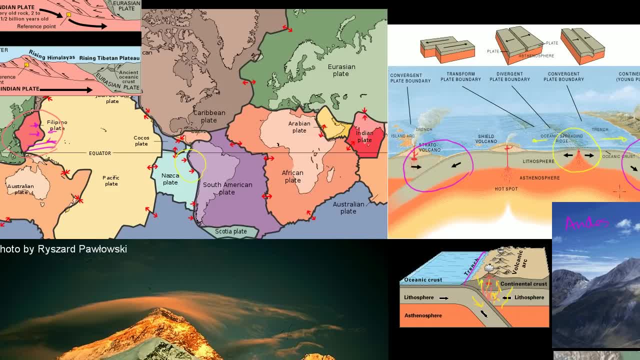 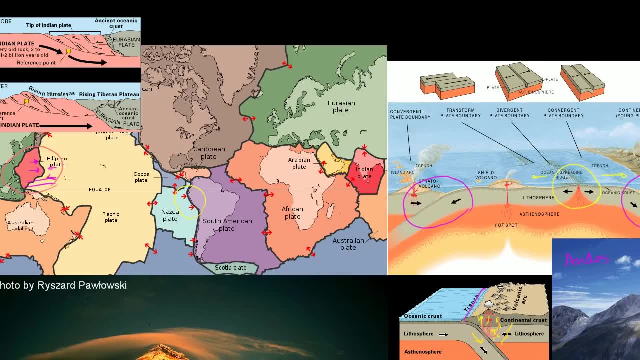 i think you might already guess what's going to happen there when you have two pieces of continental crust running into each other. one isn't more or less dense than the other, and so at least the crustal portions of them, the crustal portions of them, are just going to keep, are just going to keep jamming into each other, and so they're just 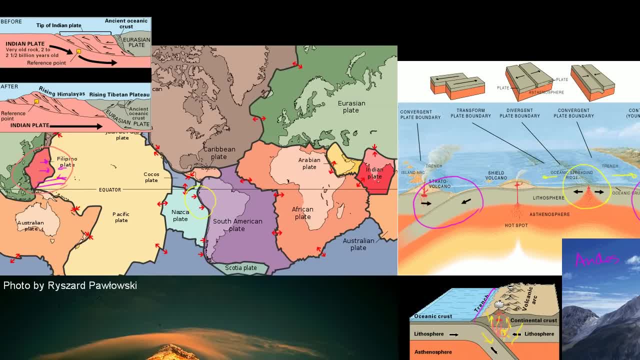 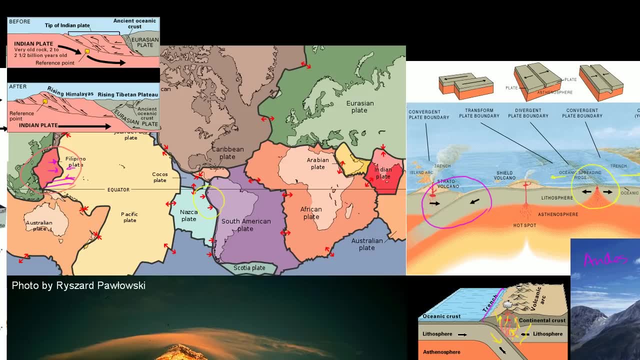 going to push things upward. this is a depiction right here that i got from the usgs and what's? what's kind of depicting is? this is the indian plate. this is the eurasian plate. this is if you, if you rewind a good bit before they've really had a chance to jam into each other. 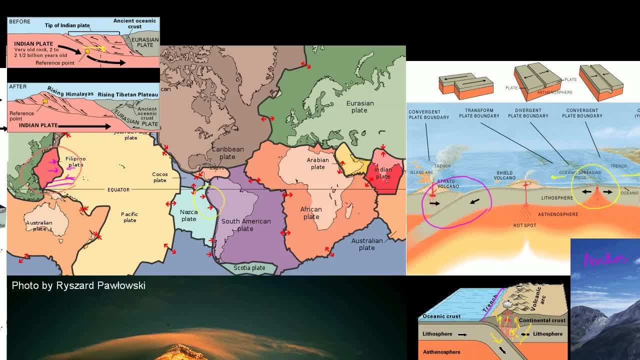 but as they're jamming into each other, the indian plate is kind of digging in a little bit, not being fully subducted, and it's causing the land to rise, and what that essentially ends up with is you end up with something like. you end up with something like the himalayas, and this right here is a. 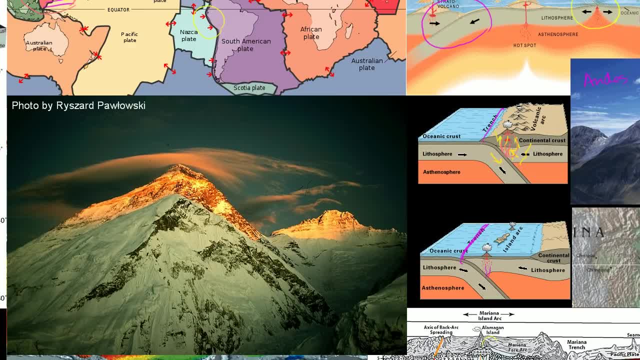 picture of mount everest, which is almost nine thousand meters high, nine thousand meters above sea level, so it's almost as high as the mariana trench is deep. 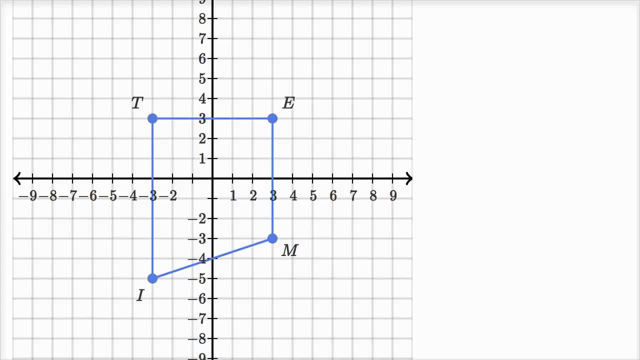 What I hope to introduce you to in this video is the notion of a transformation. in mathematics- And you're probably used to the word in everyday language, transformation means something is changing, It's transforming from one thing to another. So what would transformation mean in a mathematical context? 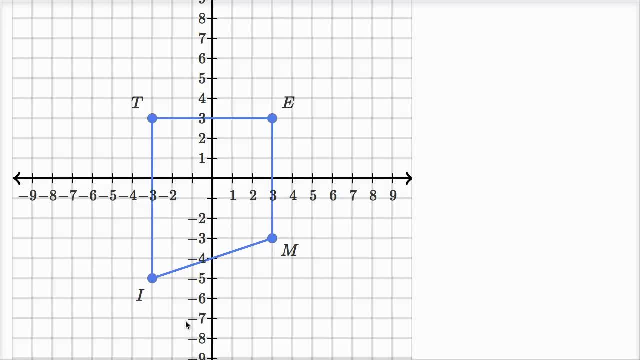 Well, it could mean that you're taking something mathematical and you're changing it into something else mathematical, and that's exactly what it is. It's talking about taking a set of coordinates or a set of points and then changing them into a different set of coordinates. 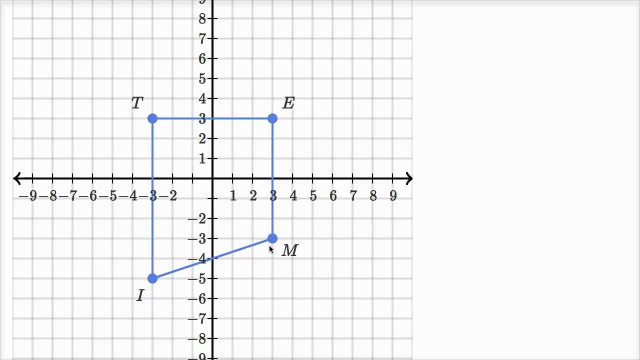 or a different set of points, For example, this right over here. this is a quadrilateral. We've plotted it on the coordinate plane. This is a set of points, not just the four points that represent the vertices of the quadrilateral.